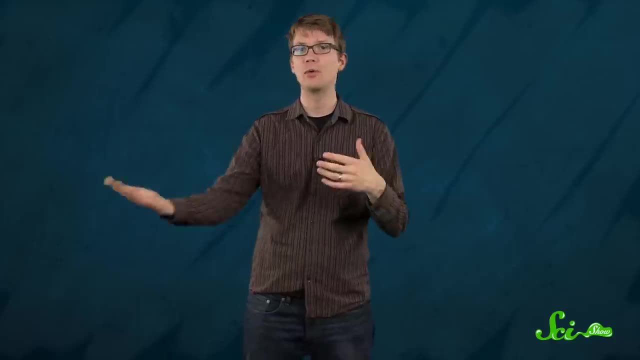 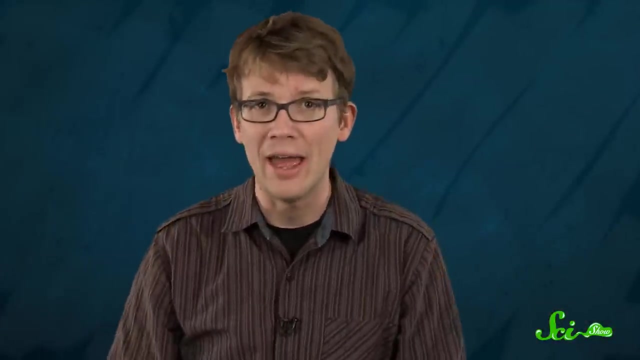 iron is eager to surrender. So when exposed to oxygen, either in air or water, the iron rusts and becomes iron oxide. So what does that have to do with burning? Well, that is a chemical reaction called oxidation. And burning is also oxidation, just much faster. So rusting is a kind of burning. It actually does give off a little bit of heat. It's just very slow and doesn't actually ignite anything. But iron can ignite under the right circumstances. The hotter that iron- or really any metal- gets. the greater its affinity for oxygen becomes. So if you get small enough pieces of it, hot enough, it'll reach a point where it undergoes what's basically very rapid oxidation. This point is its ignition temperature. You can try it at home. All you need is some extra fine steel wool, some pliers and like. 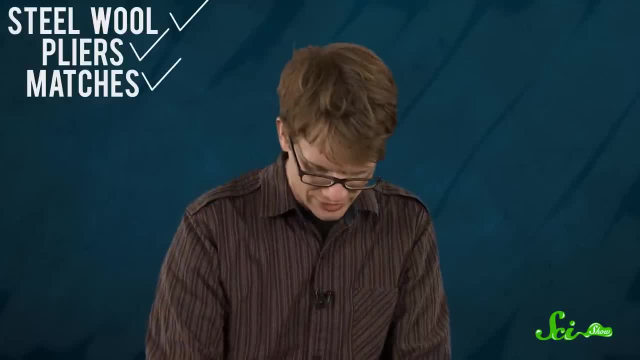 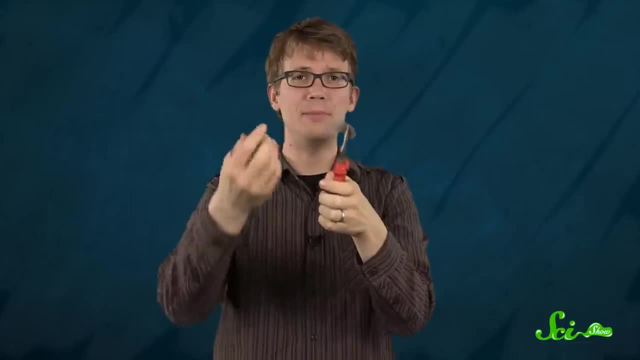 a lighter or something that makes fire and something that you can catch the hot flakes of metal in, So that they don't fall on your counter and catch your house on fire. Be careful. This steel wool is basically just thinly shaved metal. It's mostly iron, and the more fine. 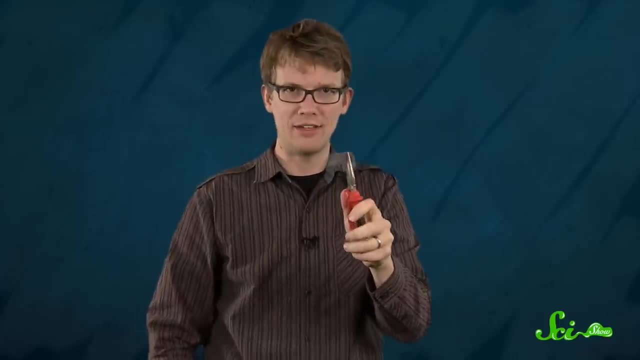 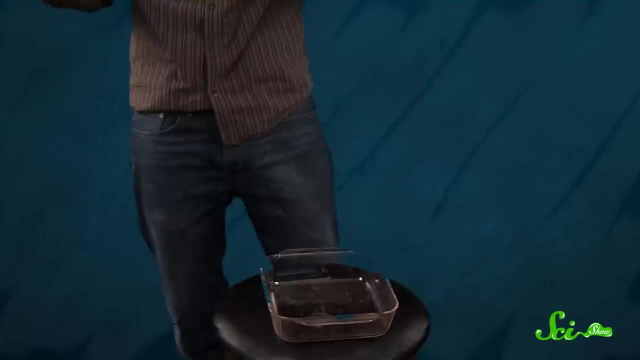 the more surface area the metal has, the easier it is to burn. Let's see if we can make this happen. Oh wow, that's pretty. It works. And did it hit me in the face with a little bit of pain? Yes, 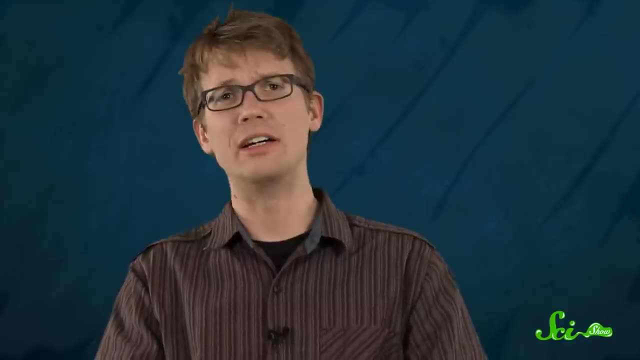 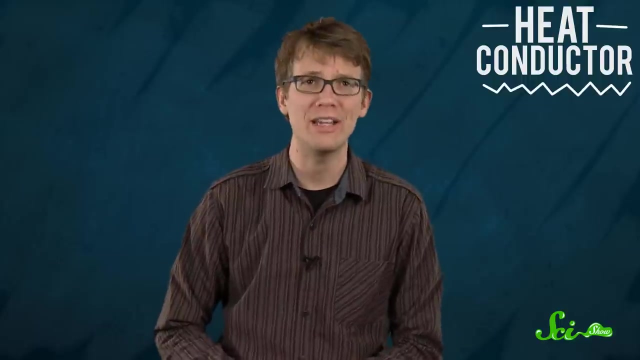 So why will steel wool burn but not the Brooklyn Bridge or a cast iron skillet? Well, for a few good reasons. First, because metal is such an excellent heat conductor. it disperses heat that's applied to it, which makes it harder for any particular part of it to reach its ignition temperature. 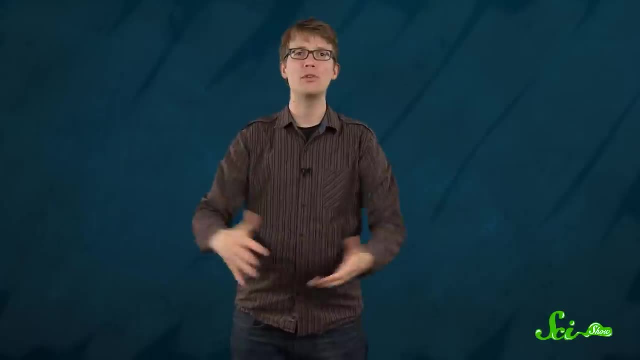 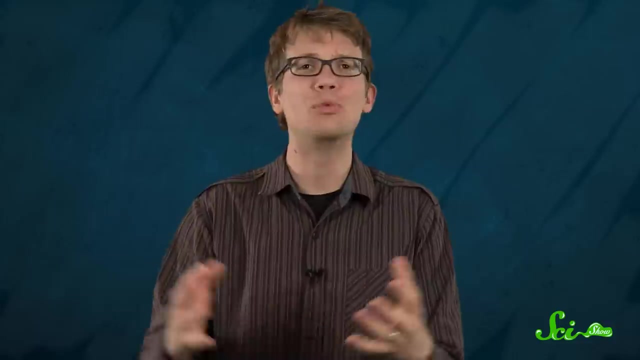 Put a skillet on a flame and the heat quickly disperses through all of the metal, so the surface doesn't get hot enough to sustain a reaction that would actually set the whole skillet on fire. But those tiny little threads of steel wool are so thin that there isn't any room for. 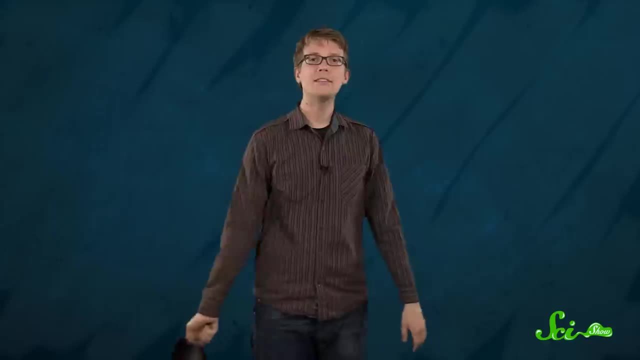 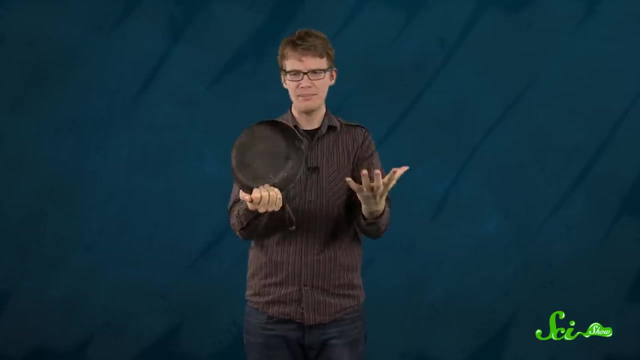 the heat to spread out, so the iron quickly reaches its ignition temperature. A second major factor has to do with surface area. Most of the iron in this skillet is inside the skillet. It doesn't come into contact with the air. Steel wool burns because these long strands have huge surface areas that are exposed and 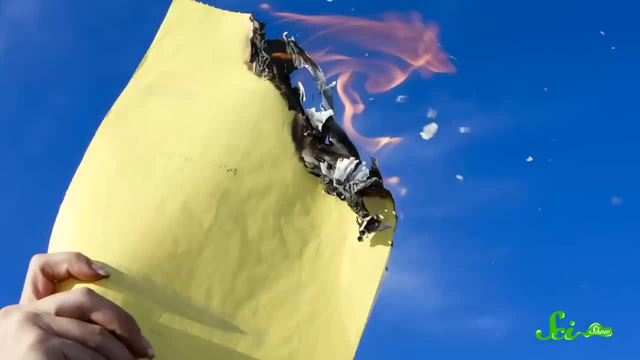 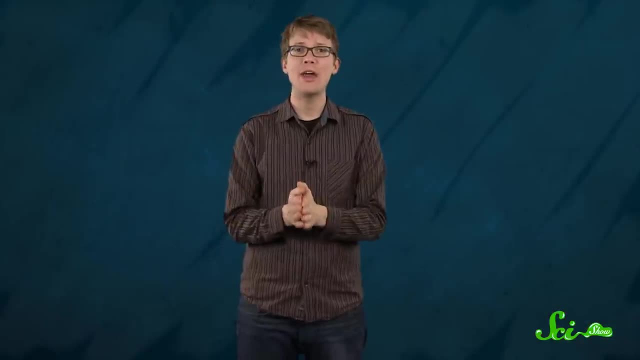 ready to react with the oxygen in the air. It's like a piece of paper is super easy to light on fire, but a big ol' log is hard to get going. Iron filings will burn, iron rods will not. In the end it's a good reminder of how everything boils down to particles, either reacting or 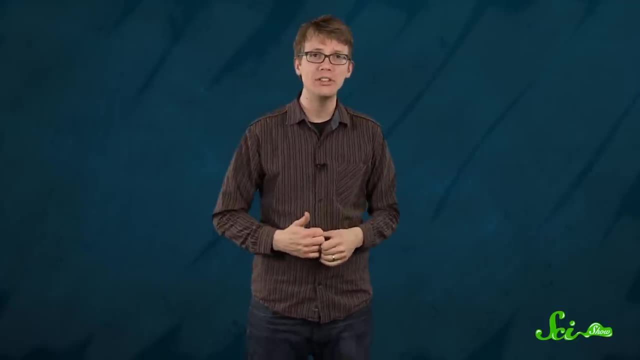 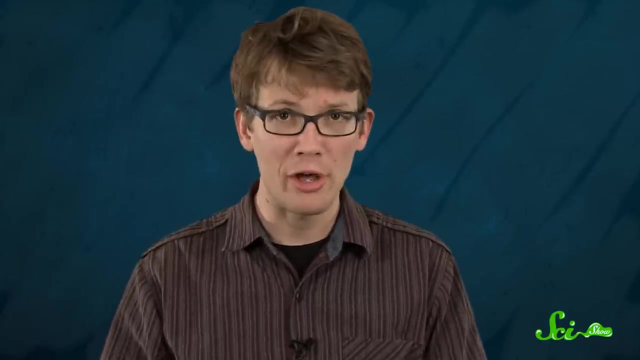 not reacting. When you visualize metal as a cast iron skillet, you only see it deflecting flames and never actually burning. But if you think of it in its elemental state and remember how iron and many other metals have big ol' crushes on oxygen, it'll broaden your understanding of pretty much anything.